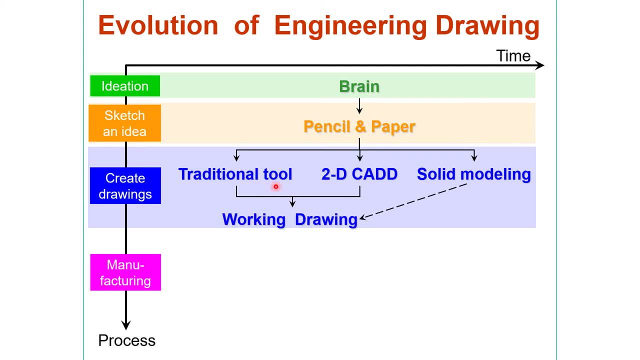 Combined with these traditional orthographic drawings and autocad drawings. Then it is given to the manufacturer a manufacturing conventional machine that is created by manual operator, that is a lathe machine, And there is also for the manufacturing of parts. there is latest technology, that is CNC machine, computer controlled machine. 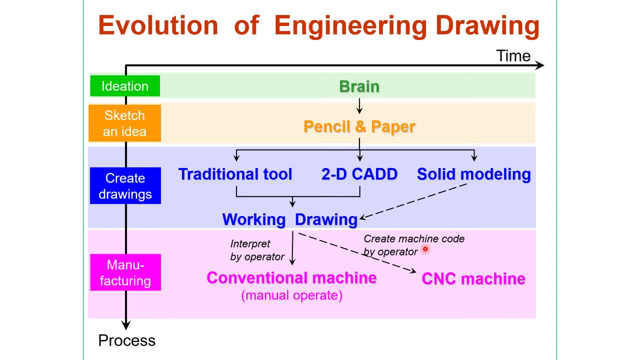 Okay, That is interpretive. So machine made by operator, by person. create machine called by operator. that is done by computer. So machine make the model. So after: at the end we got the parts as per our design needs. 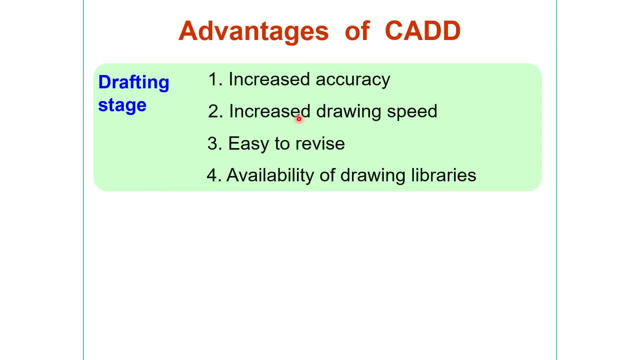 Advantages of CAD: Increase accuracy. Increase drawing speed. Easy to revise Means. if there is any mistake, we can just with the computer As the lead. the line will be deleted. Easy to revise. Availability of drawing library: There is already built in library like washrooms, sink basins, free sofas, bedroom. 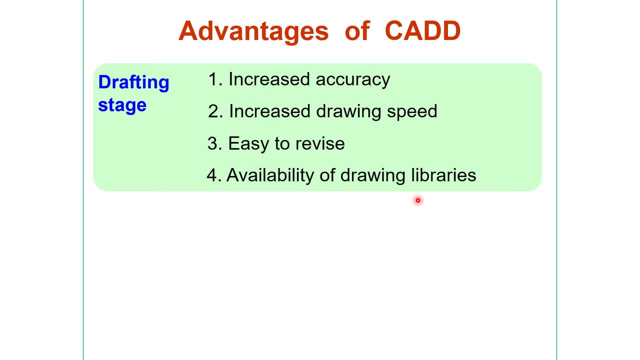 All the library almost are already present in the autocad So that is easy to use. Design stage Building several analysis tools, Like after making a geometry. with Uh, A single command of area, You can measure the area, so better presentation. 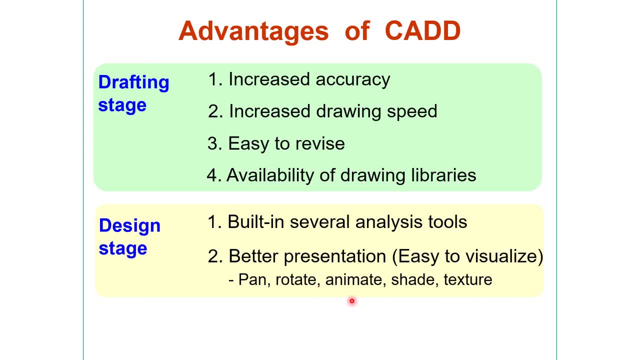 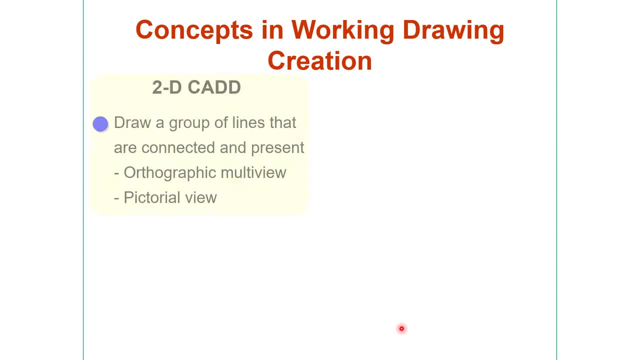 Easy to visualize. then we can rotate the model, animate shade and texture Concepts in working drawing creations. 2D drawing, 2D CAD draw a group of lines that are connected and present orthographic, multi views, pictorial views. 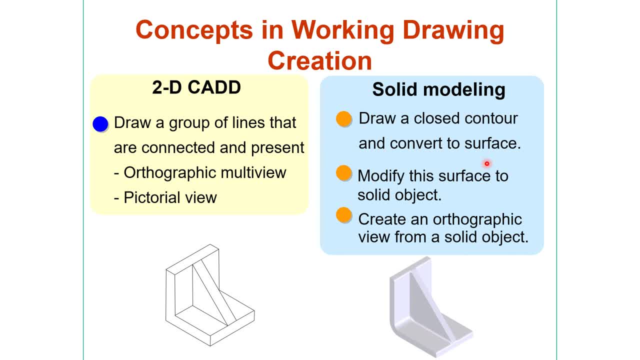 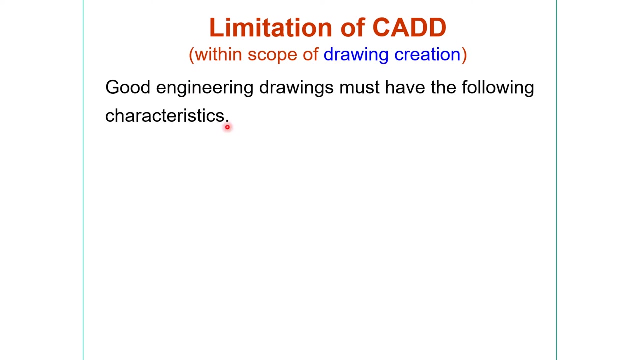 And in the solid geometry, when we make the models draw A closed contour and convert to surface, modify this surface to the solid object. create an orthographic view from a solid object. that can be done in the 3D drawing in the CAD- limitation of CAD within scope of drawing creation parts or products. 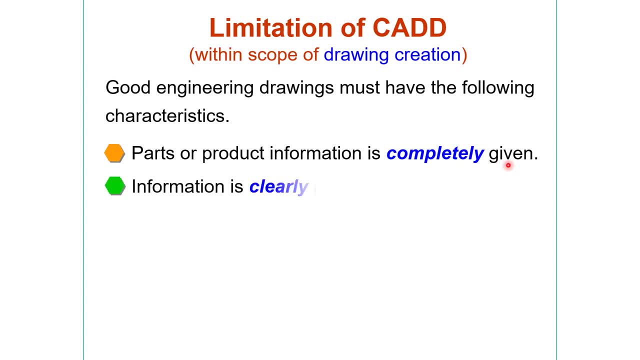 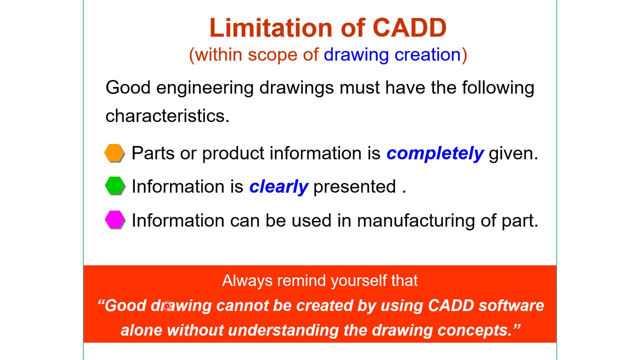 Information is completely given. Information is Clearly represented. Information can be used in manufacturing of art. That is a good reminder. Always remind yourself. Good drawing cannot be created by using CAD software alone. It is with the help of CAD only. You cannot make the good drawings without understanding the drawing concepts. 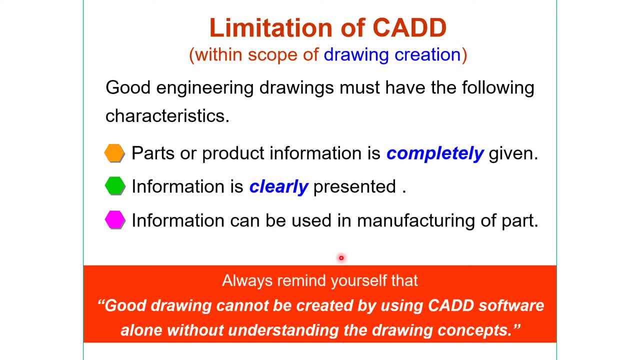 If you do not know what is center line, hidden line, how to make With the help of CAD software, you cannot make the good drawings. So how to show the hidden features. So if you do not know that drawing concepts, you cannot make the good drawings. 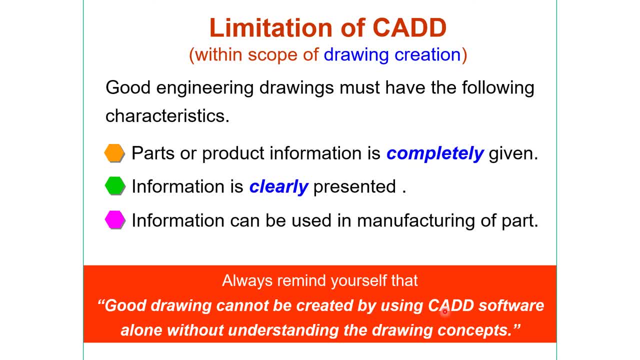 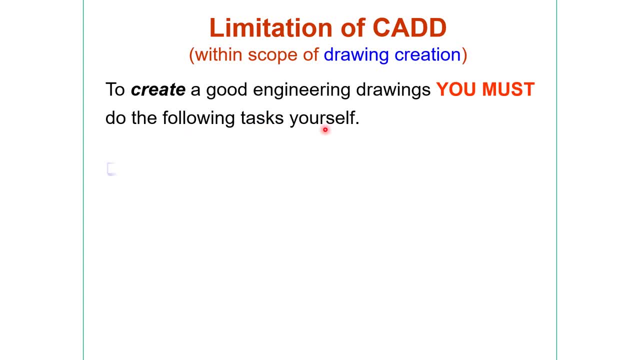 So far. making of good drawings. You should know drawing concepts and also CAD. To create a good engineering drawings, you must do the following tasks yourself: Apply a proper line width and style means what will be the thickness. Select a necessity view which will 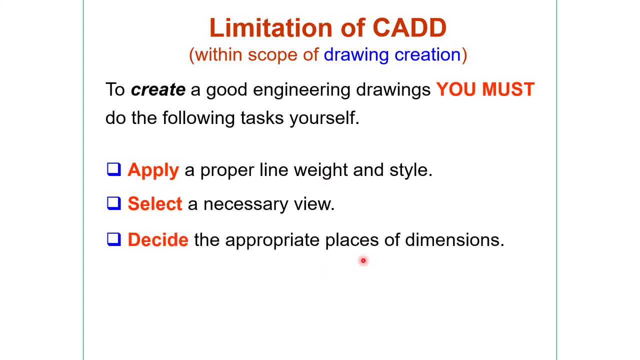 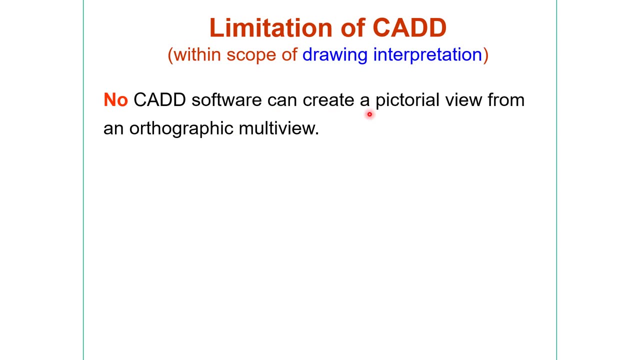 New will be necessary. decide the appropriate place of dimensions where dimensions will be placed. select an appropriate section- techniques, if that is necessary. section views: limitation of cad. no cad software can create a pictorial or 3d view from an orthographic view or multi-view automatically. 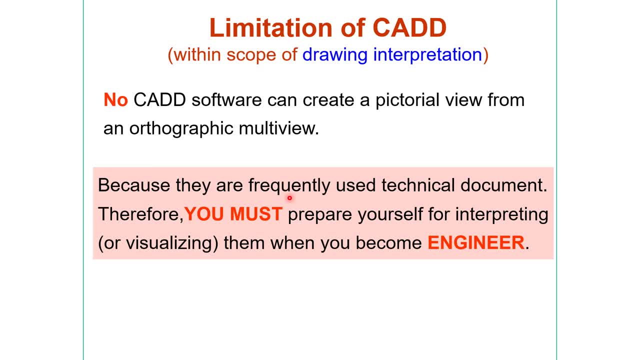 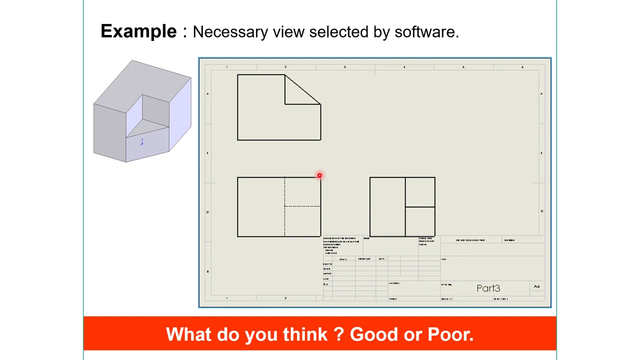 because they are frequently used technical documents. therefore, you must prepare yourself for interpreting or visualizing them when you become an engineer. so that is your responsibility. to how to rate the orthographic or multi-view drawings to visualize the 3d object, that is your responsibility. now here is a brief demonstration of the drawings in the drawing sheet. so here is. 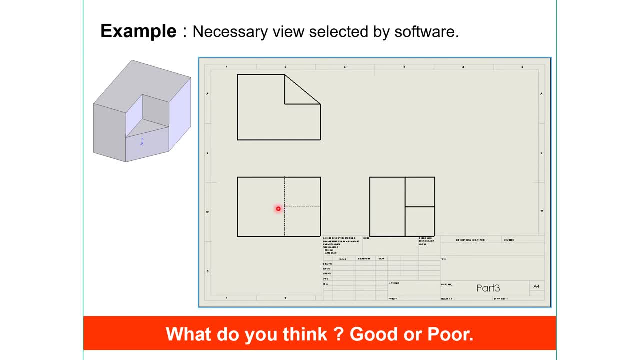 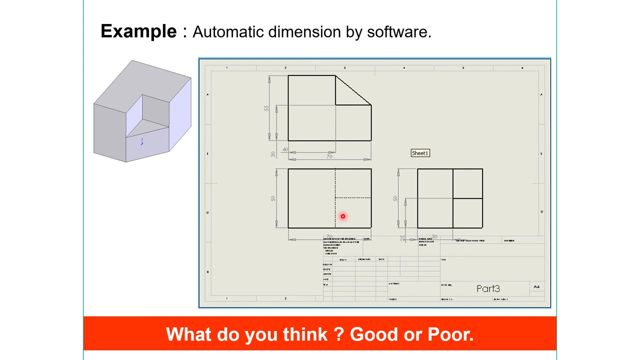 the top view of front view view, uh, you can say that is from the behind, that is rear view and the side view. so, but in this drawing there is a one disadvantage: that there is no detailing. so the second one, the top view. uh, whatever the drawing is shown, uh, top view. okay, so here is the top view. so if you see from this,